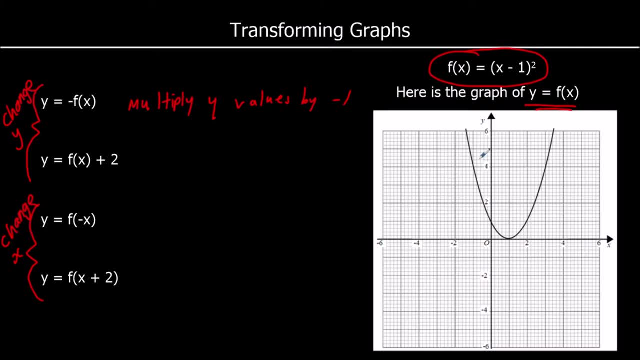 let's have a look at how that looks. So there's, we had negative 1, 4.. That's going to become negative 1, negative 4.. 0, 1 would become 0, minus 1.. 1, 0 would stay as 1, 0.. 2, 1 would. 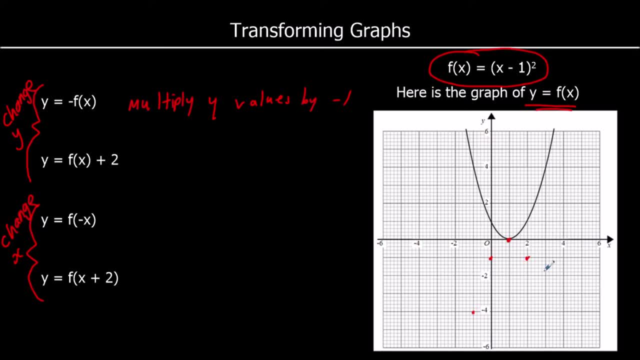 become 2, negative 1.. 3, 4 would become 3, negative 4.. So what this graph looks like is a reflection in the x-axis. So I'm going to write reflection, reflection, Reflection in x-axis. So y equals minus f of x. It changes the y-coordinates, So we're 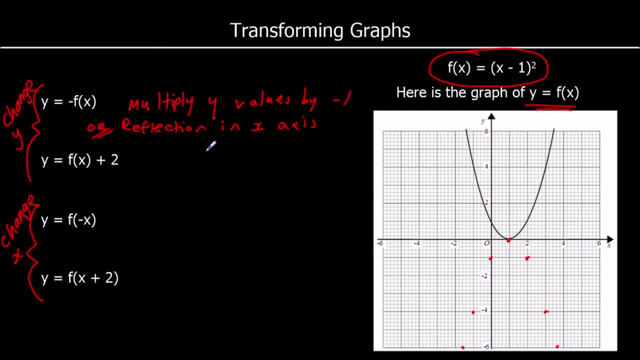 multiplying all the y values by negative 1.. Or it's a reflection in the x-axis: For y equals f of x plus 2, for y equals f of x plus 2, we're going to add 2 to all the y. 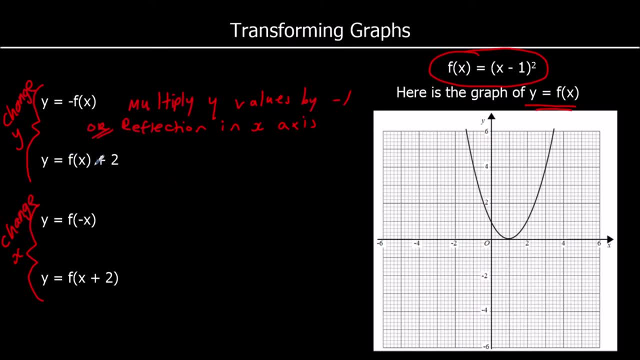 values, So 0,, 0,. whatever we get out of the function, we're going to add 2 to it. So where we got out 0 before, we're going to shift it up. 2 spaces: Where we had 1, we're going to shift it up. 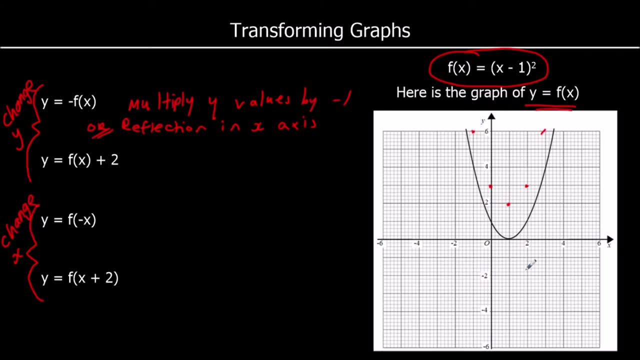 2 spaces, So this whole graph is shifted up. 2 spaces. So for f of x plus 2, we're going to add 2 to all the y values, all the y coordinates. If it was f of x minus 2, we're going to add: 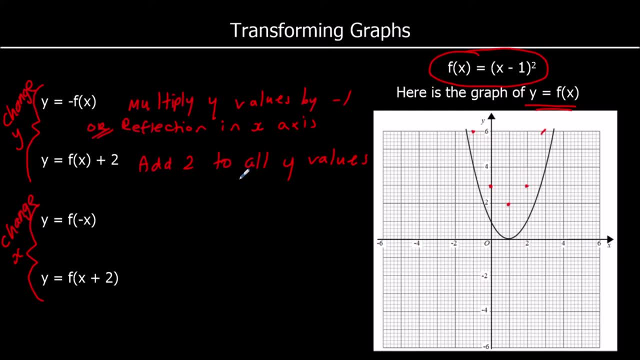 2. It would move down. 2. We'd take 2 away from all the y coordinates. If it was f of x plus 7, it would move up 7 spaces. We'd add 7 to all the y coordinates. So they are the changes. 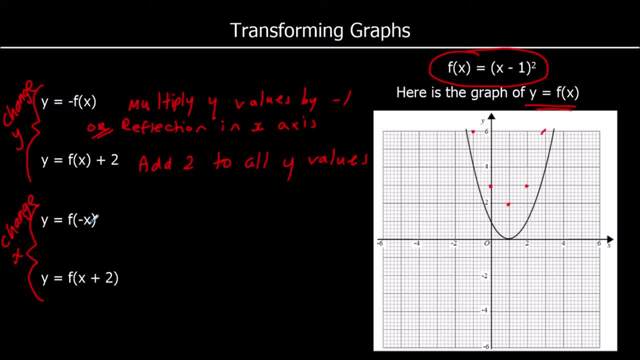 to the y. we need to know The changes to the x. For y equals minus, for y equals f of minus x. we multiply all the inputs by negative 1. So if we put in negative 2, that will be the same as the original 2. If we put in 5, that 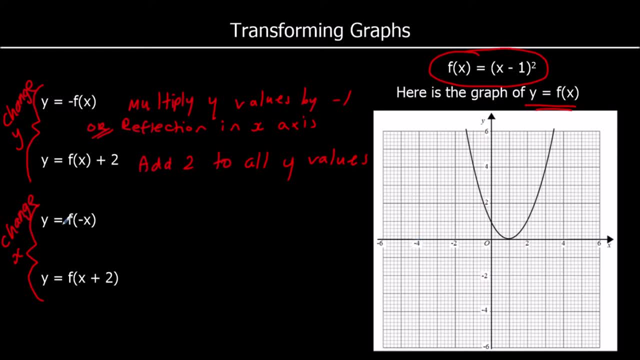 would be the same as the original negative 5.. So this transformation multiplies all the x coordinates, all the x values by negative 1.. So where we had 1, 0,, that becomes negative 1, 0.. 0, 1 will stay where it is. Where we had 2, 1,, that becomes negative 2, 1.. 3, 4. 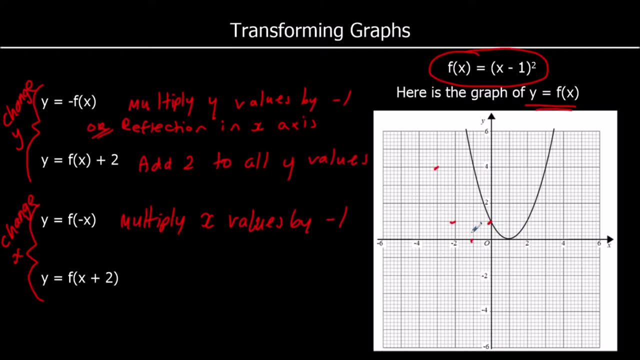 will become negative 3, 4.. Negative 1, 4 will become positive 1, 4.. So we're multiplying all the x values by negative 1, and that looks like a reflection In the y-axis. So I'm going to graph that will look like a reflection in the y-axis. 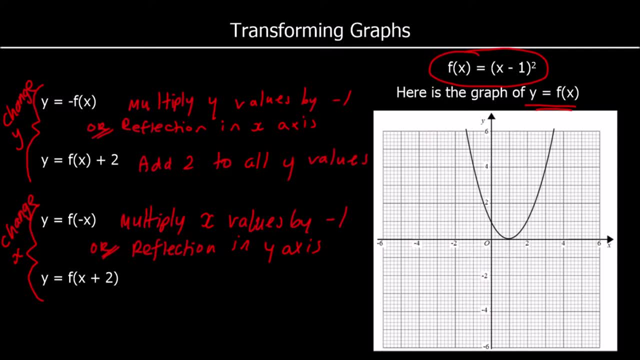 And how about the last one? y equals f of x plus 2.. So there are changes inside the bracket, so we know it's going to change our inputs, our x's. Let's look at what would happen if we add 2 to our input. So where we put in. if I put 0 into this function, it's. 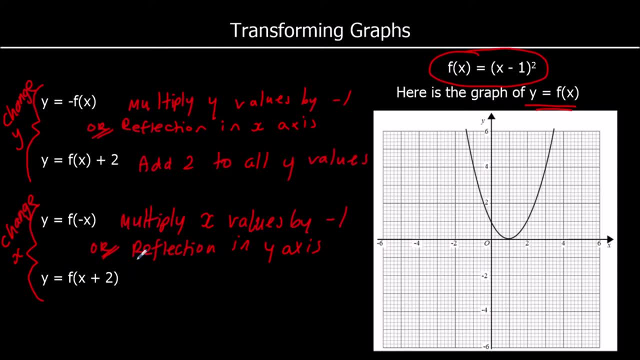 going to behave like it is 2, because you're adding 2 to it. So if I put in 0,, I'm going to get the answer out for 2.. If I put in negative 1,, I'm going to get the answer out for 1.. 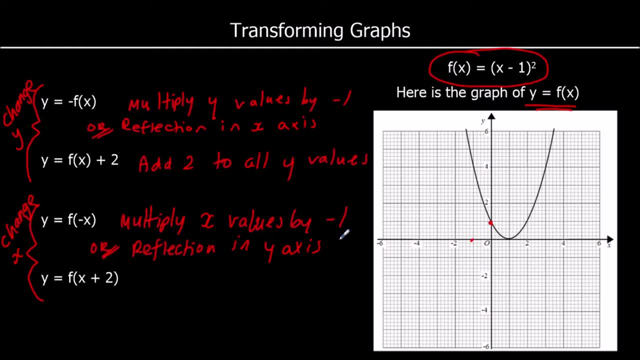 If I put in negative 2, I'm going to get the answer out for 0.. If I put in negative 3, negative 3 plus 2 is negative 1, I'm going to get the answer out for negative 1. so it's shifting 2 spaces. 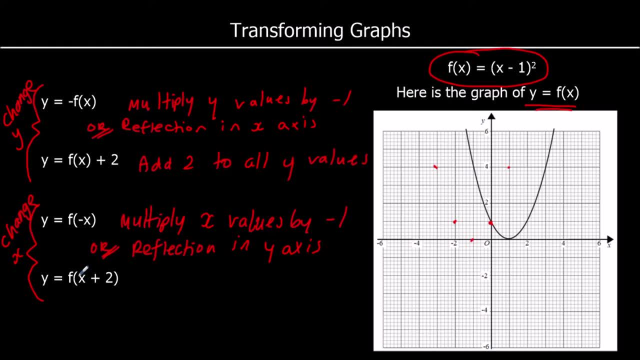 to the left. so f of x plus 2 subtracts 2, takes 2 away from the x coordinates. so f of x plus 3 will take 3 away from the x coordinates. if I had f of x minus 2, I would actually add 2 to the x coordinates. 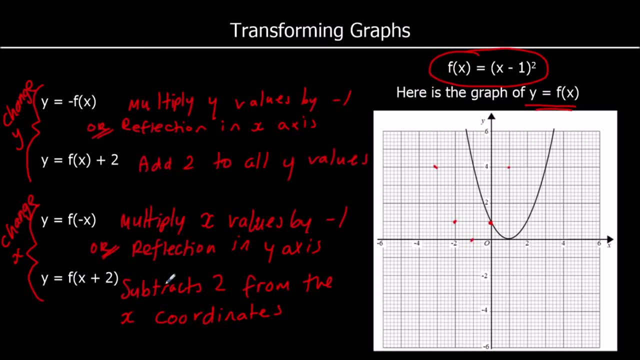 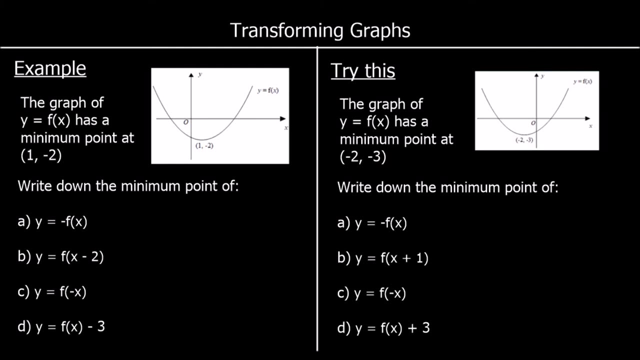 so it does the opposite to what it says. if you have f of x minus 7, you add 7 to the x coordinates. if you have f of x plus 1, you take 1 from the x coordinates. ok, let's look at a question. the graph of y equals f of x. 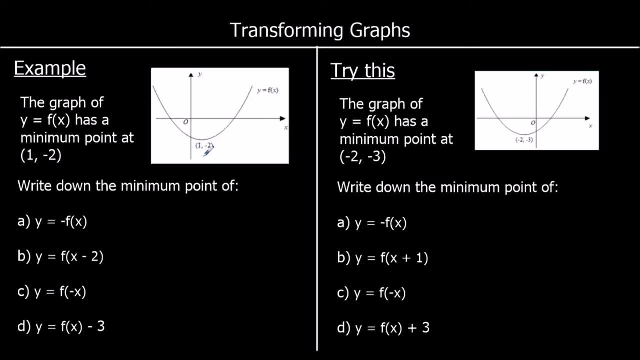 has a value of 3. there's a minimum point at 1, negative 2. so x is 1, y is negative 2. write down the minimum point of. so the first one, y equals minus f of x. so we can see the change is outside of the bracket. 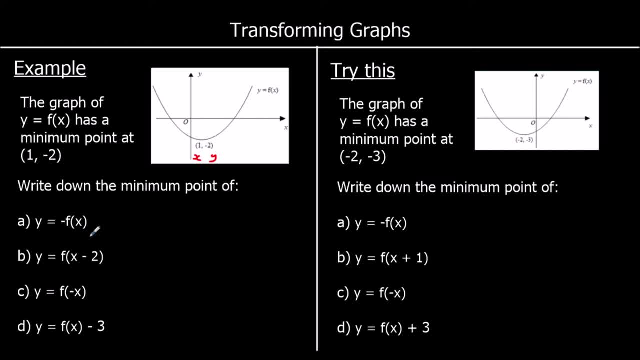 it's changing the y, it's outside the bracket, it changes the y and we're going to multiply the y by negative 1, so we're going to leave the x as it is and negative 2 times negative 1 is 2, the second one. 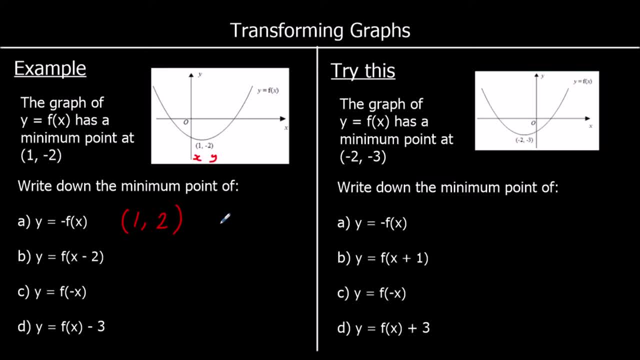 y equals f of x minus 2. the change is inside the bracket. it changes the input, changes the x and it does the opposite. so it says x minus 2. we're going to add 2 to the x coordinate, so it's going to become 3 negative 2. 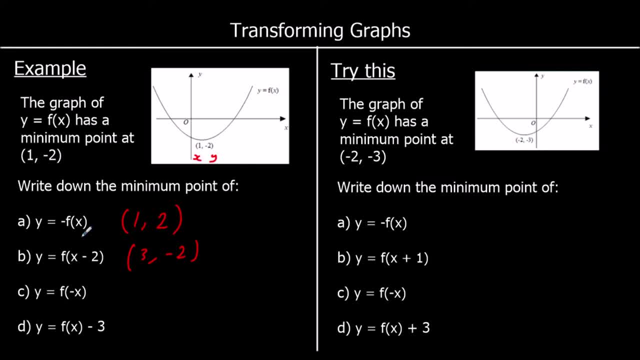 we leave the y alone and we change the x coordinate. we change the x. for the third one, y equals f of minus x. so we're changing the x. the change is inside the bracket, and we're going to multiply the x by negative 1, so that becomes negative 1. 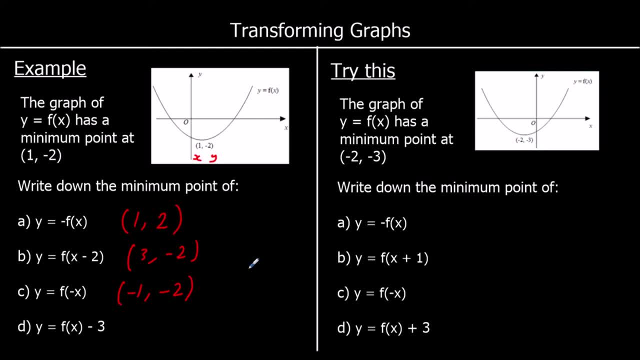 negative 2 and the last one, f, of x minus 3. the change is to the y and we're going to take 3 away from it, so the graph shifts down 3, and that leaves us with the y prime and y 2, which is monopolized. 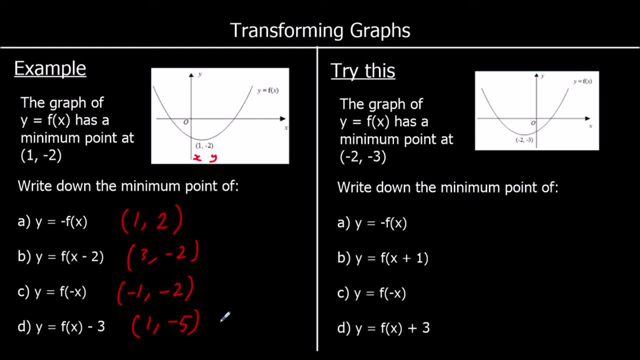 because we're not going to multiply now femton minus 3 for that equation. 3th power, 3, union cost f of x minus 3, x minus 3. so we've given it a term, f of x minus 2, and we're going to multiply it each time. 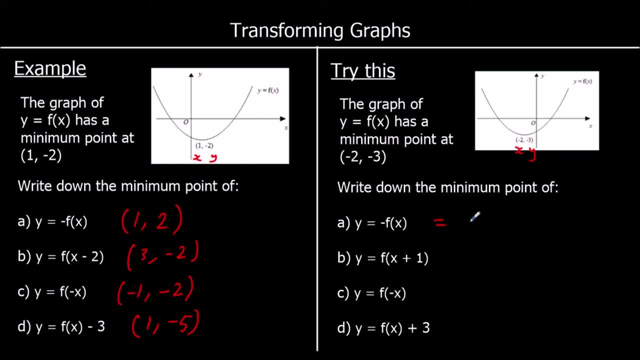 1. It's a reflection in the x-axis, so that'll become negative 2,. 3. y equals f of x plus 1, so it's inside the bracket. It changes the x, and if we plus 1 inside the bracket, 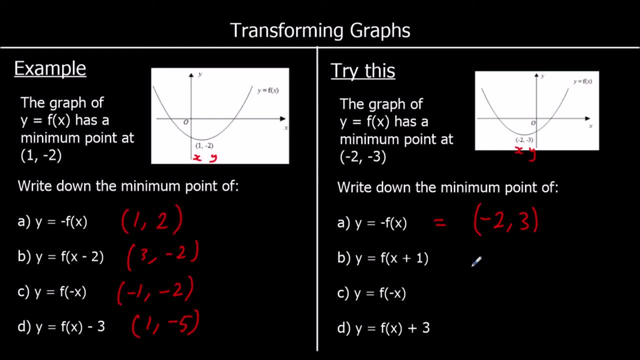 that means we're going to take 1 away. It does the opposite, so it'll go to negative 3, negative 3.. We leave the y alone and change the x. y equals f of minus x. so again we're changing the x, we're leaving the y alone and it multiplies the x by negative 1.. 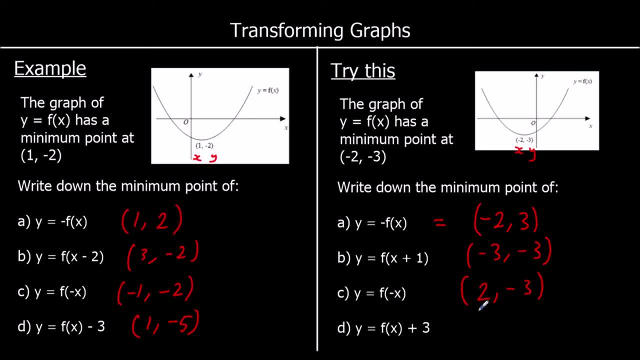 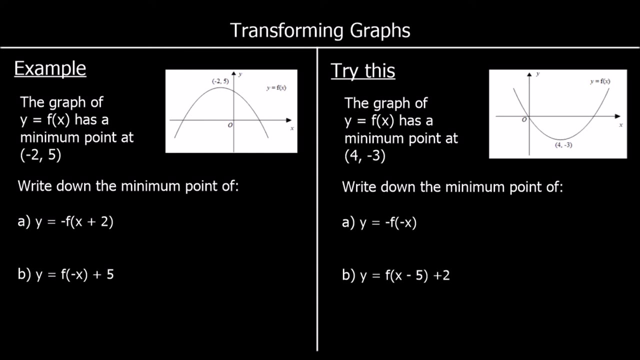 And f of x plus 3, so we leave the x alone, we're changing the y and we're adding 3 to it. So negative 3 plus 3 is nothing. Okay, here's an example where we have two transformations going on. So we're going to. 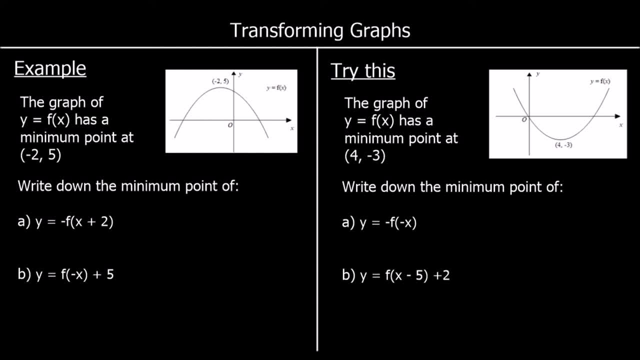 have one transformation for the x and one for the y. So we've got a graph with a minimum point of negative 2, 5, and we want to know what happens when we transform it into the graph minus f of x plus 2.. So for the x coordinate we're going to take 2 away. 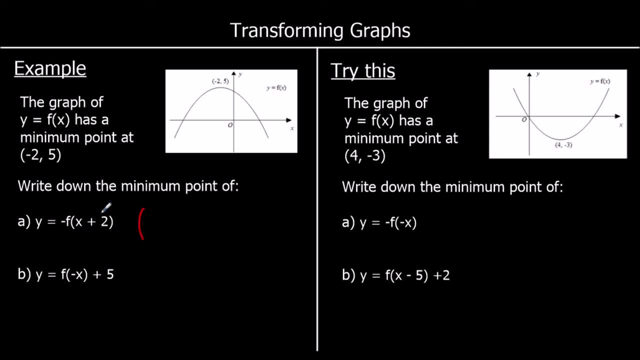 so inside the bracket changes the x and we're going to do the opposite. So we're going to take 2 from the x, so that'll become negative 4, and we're going to multiply our y by negative 1, so that becomes negative 5.. For b, we're going to multiply our x by negative. 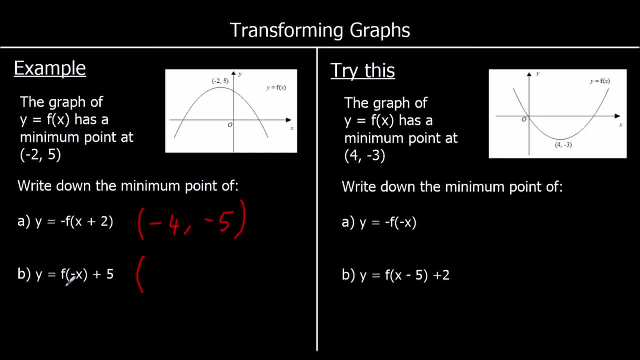 1. The change inside the bracket is to multiply x by negative 1, so that becomes 2.. And the change to the y is a plus 5, so 5 will go up to 10.. Okay, one for you to try. so give this a go. 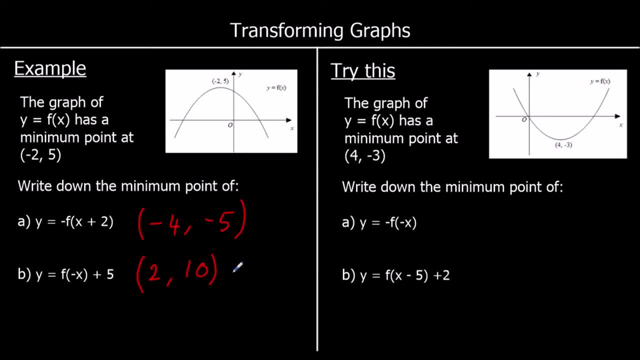 Okay, so we're starting off with a minimum point of 4, negative 3, the first graph is: y equals, or the first transformation: y equals minus f of minus x. So it flips. it reflects in the x-axis and the y-axis. 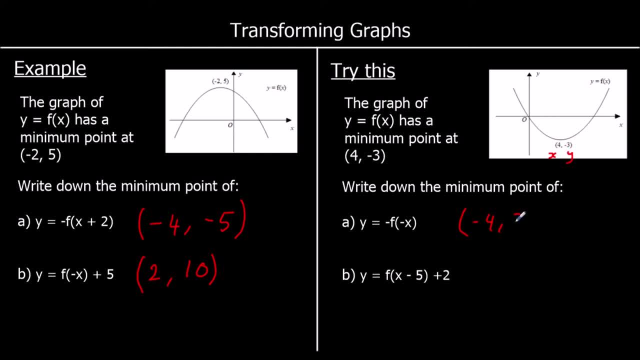 so we multiply the x coordinate by negative 1 and the y coordinate by negative 1.. y equals f of x minus 5 plus 2, so we're going to add 5 to our x and we're going to add 5 to our y coordinate. so it does the opposite inside the bracket. 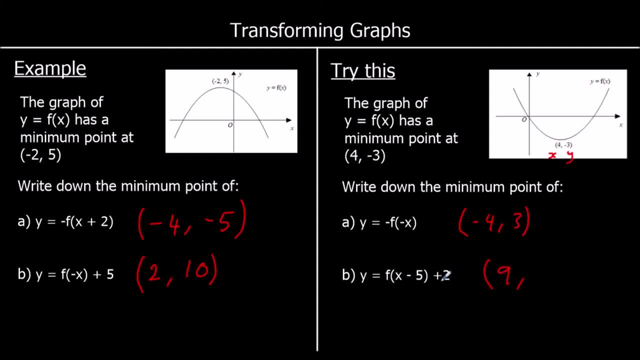 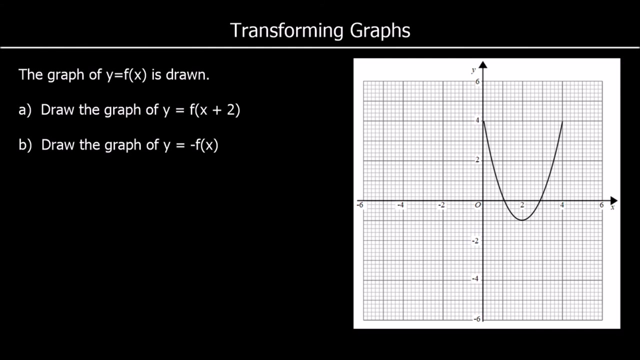 so that becomes 9.. And we're going to add 2 to our y coordinate. so negative 3 goes up to negative 1.. So it shifts 5 to the right and 2. up Here we've got a graph drawn for us, so the graph is drawn on the grid. 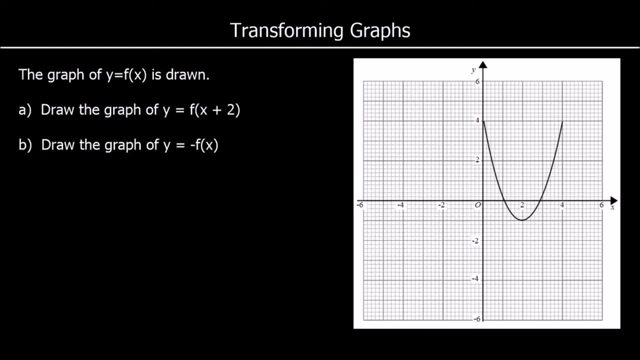 and we're going to add 2 to our y coordinate. so negative 3 goes up to negative 1.. So we're asked to draw the graph of: y equals f of x plus 2.. So f of x plus 2, the change is inside the bracket and we do the opposite. 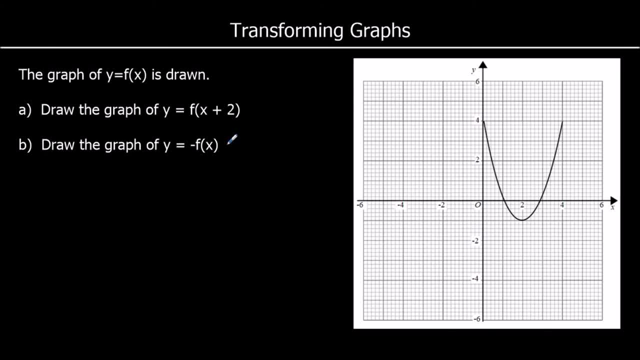 So it says plus 2, we're going to take 2 away, So we're taking 2 off all of the x coordinates. So it's going to shift 2 to the left. So it's going to look like this: 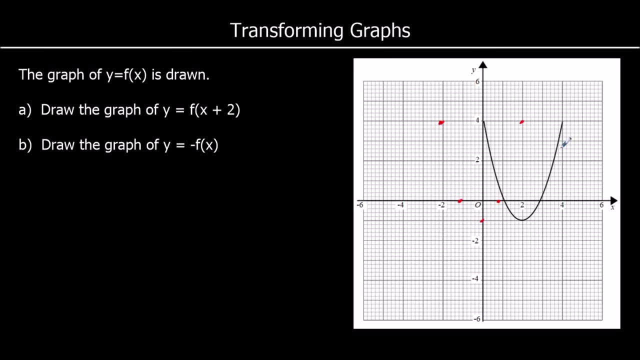 We're shifting every point 2 spaces to the left. So we've got something like this and I'm going to try and join them up. So it's something like that: How about the graph of minus f of x? So this is a change to the y coordinates. 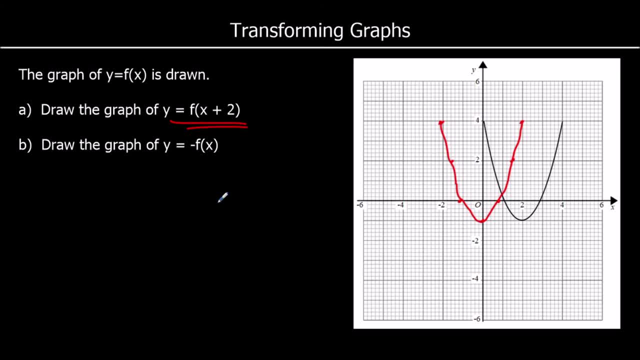 We're going to multiply all of the y coordinates by negative 1.. So it's reflecting in the x-axis: A 4 is going to become a negative 4.. A negative 1 is going to become a positive 1.. A 4 is going to become a negative 4.. 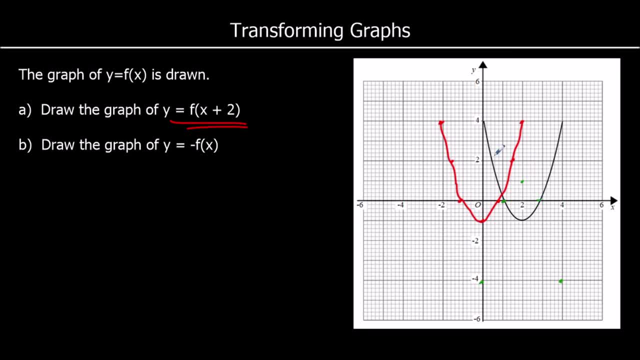 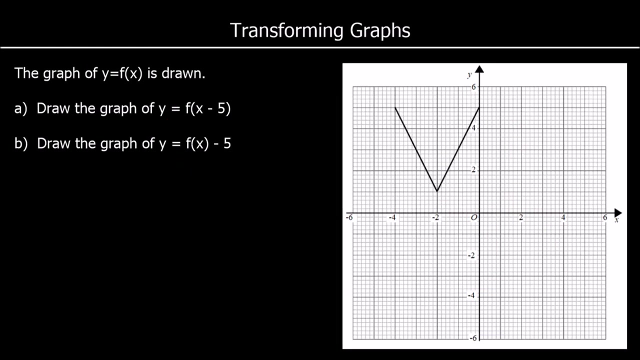 The points where it crosses are going to stay the same And we'll try and join up these points. So it looks something like that: Okay, another graph. Another graph is drawn. We need to draw the graph of: f equals x minus 5,. 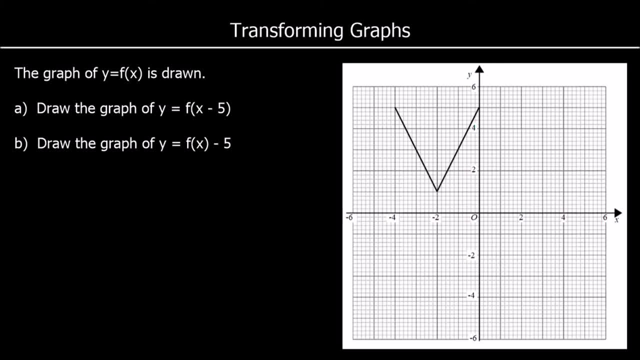 and f of x minus 5.. So the first one is a change to the x coordinates. It's inside the bracket, It changes the x And it says minus 5.. So we're going to plus 5 to all the x coordinates. 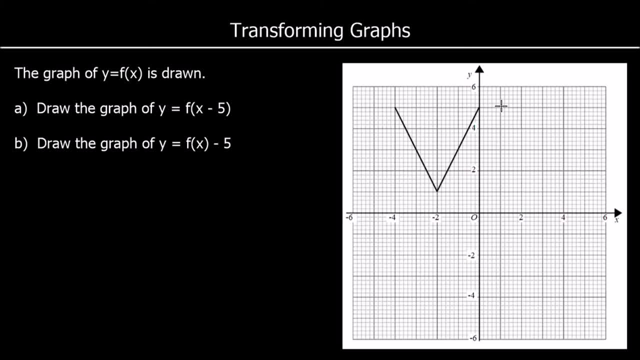 So where we had negative 4, that's going to become 1.. So it's going to shift 5.. So it's going to shift 5 spaces to the right. The graph shifts 5 spaces to the right, So it will look like this: 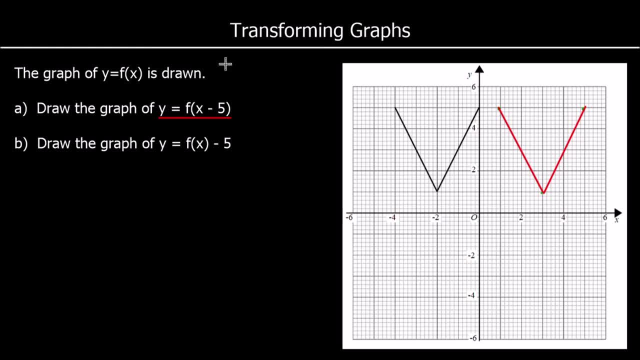 And the graph of f of x minus 5.. So this time we're going to move the whole graph down 5 spaces, So we're at 5.. That goes to 0.. 5 goes to 0.. And 1 goes to negative 4.. 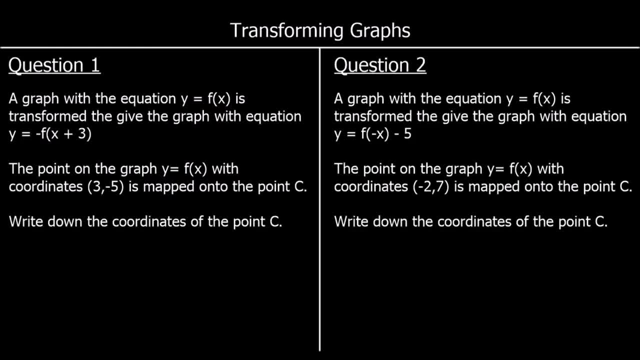 So there is our graph And to finish up, we have two questions. Pause the video, Give them a go And press play when you're ready for the answers. Okay, A graph with the equation y equals f of x is transformed to give the graph of equation y equals minus f of x plus 3.. 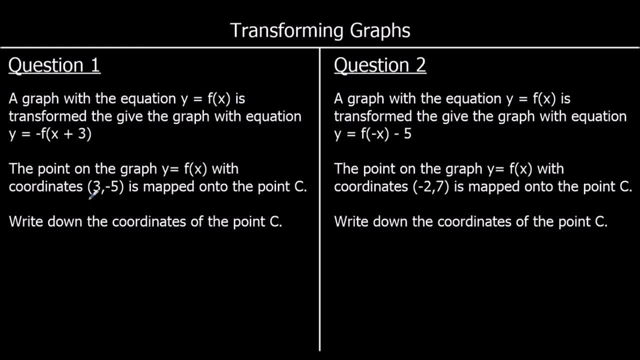 The point on the original graph with coordinates 3, negative 5 is mapped onto c. Write down the coordinates of c. So what do we have to do to these coordinates? So we're going to The x. change is inside the bracket. 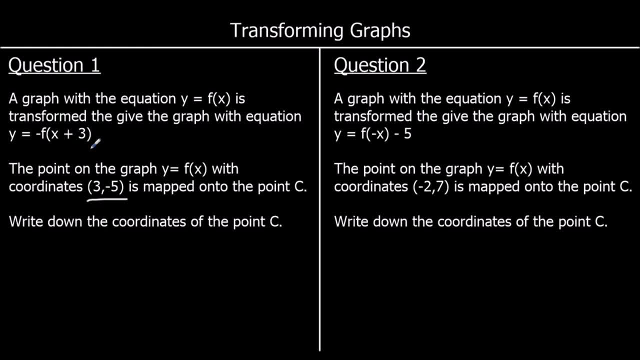 And it does the opposite. So it's z plus 3.. But we're going to take 3 away. So 3 take away 3 is 0.. And the y change is to multiply by negative 1.. So we had negative 5..